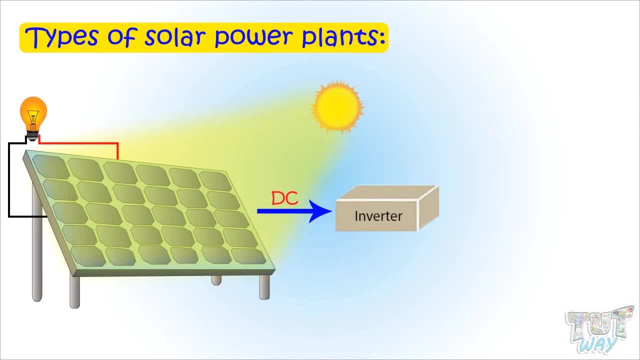 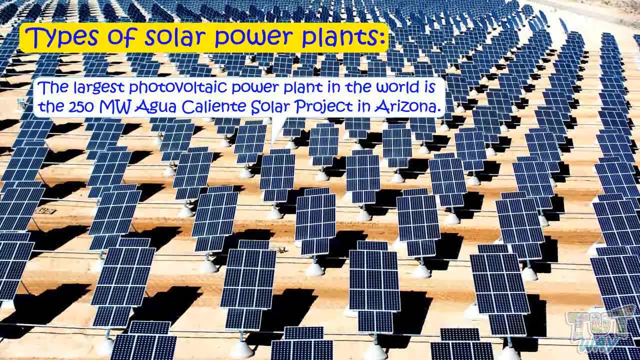 alternating current, AC or the alternating current. it is in this form that energy is supplied to homes, offices and other buildings, which we also call as electricity. the world's largest photovoltaic power plant is in Arizona. it is 250 megawatt power plant and its name is agua caliente solar. 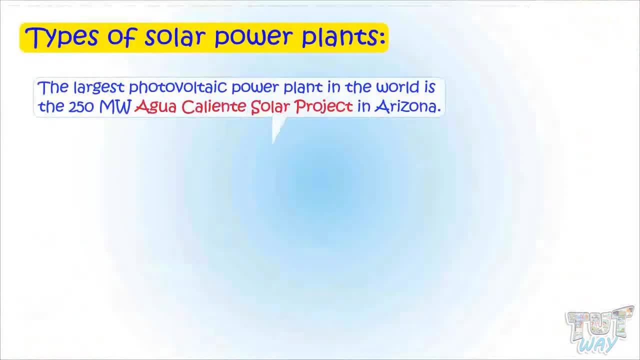 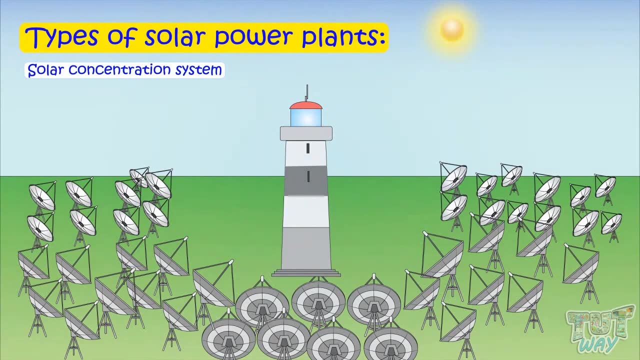 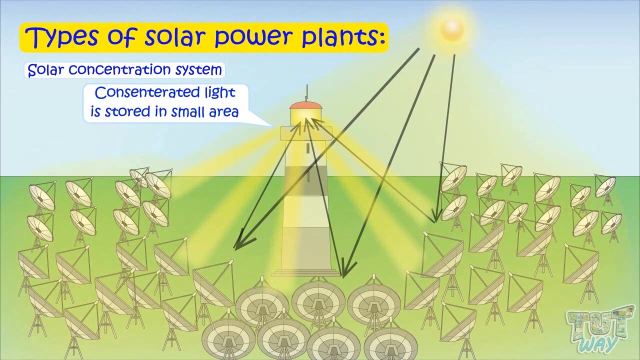 problem project. there is one more type of solar power plant, and they are known as solar concentration systems. these systems use mirrors or lenses that concentrate the large amount of light falling on a large area onto a small area, and this concentrated light on the small area produces a lot of light. 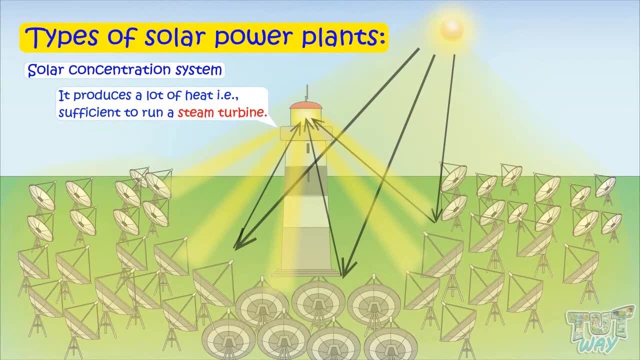 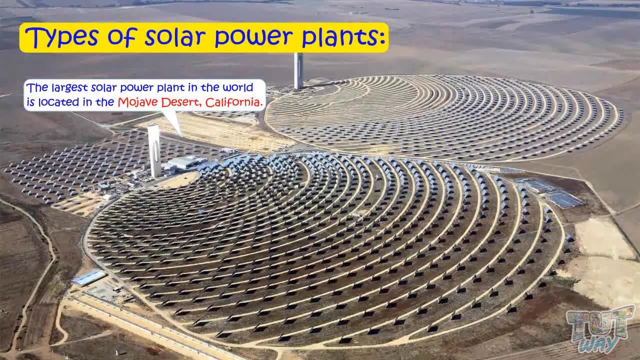 a lot of heat that is sufficient to run a steam turbine that eventually runs a generator and produces electricity. The largest solar power plant in the world is located in the Mojave Desert, California. It is a 354 megawatt solar power plant. 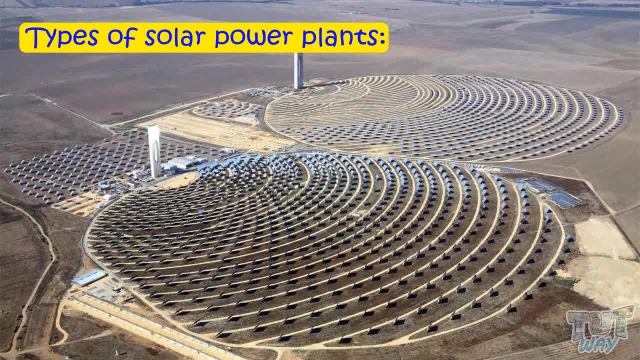 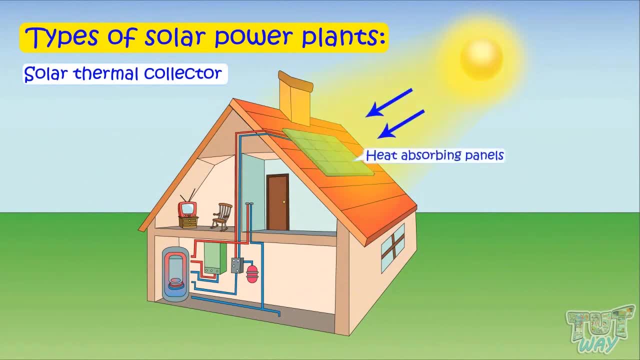 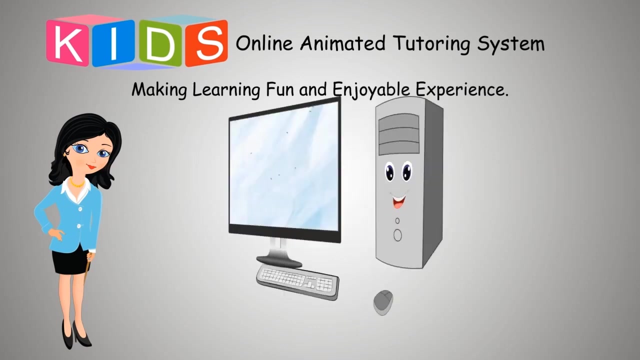 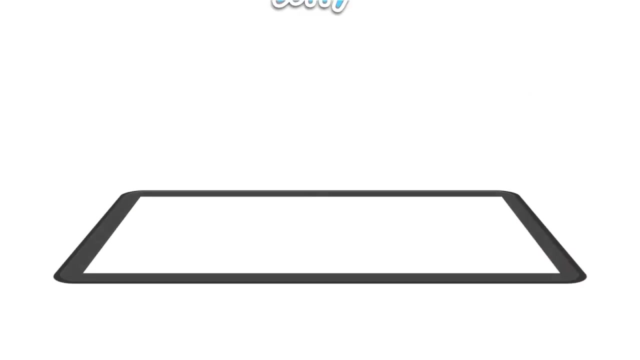 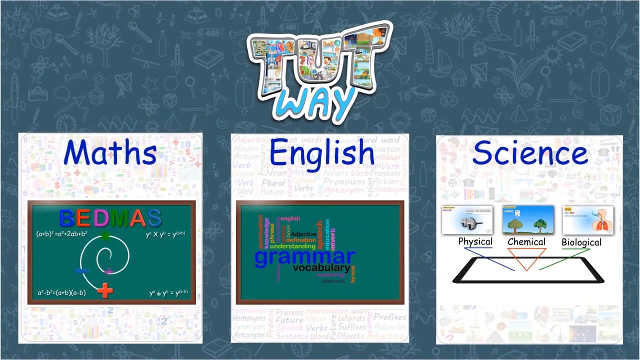 There is one more way of using the solar energy: Solar thermal collectors use the heat-absorbing panels and a series of attached circulation tubes that carry water, and this water is heated and then supplied to the buildings for domestic use. TootWay has thousands of animated videos on math, English and science to clear the 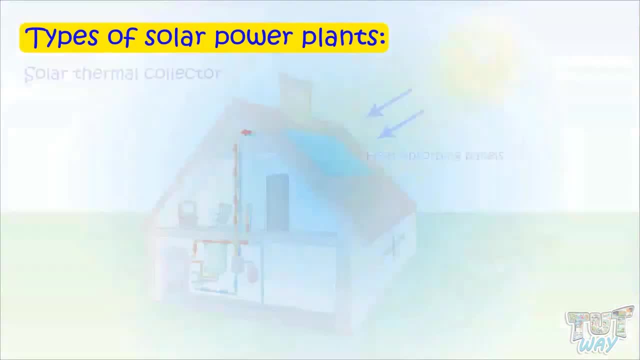 core basics of these subjects. There are a lot of many advantages of using solar energy. It is readily and abundantly available, Very affordable, A very clean source of energy, Renewable. Every country can produce its own electricity. Reduces pollution, Helps to keep the fossil fuel prices lower. 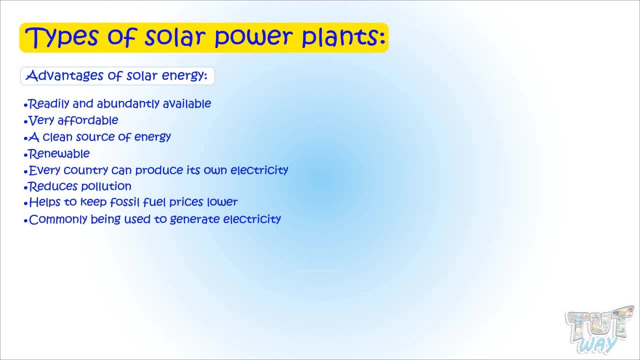 It is commonly being used to generate electricity. It is very convenient to use it in our homes For heating water using the solar water heater. Solar panels require much less maintenance. They do not have any mechanical parts that can fail. Solar energy is a resource that is not only sustainable for energy consumption, it is 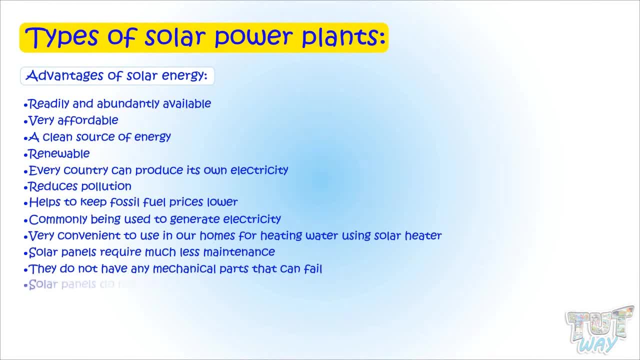 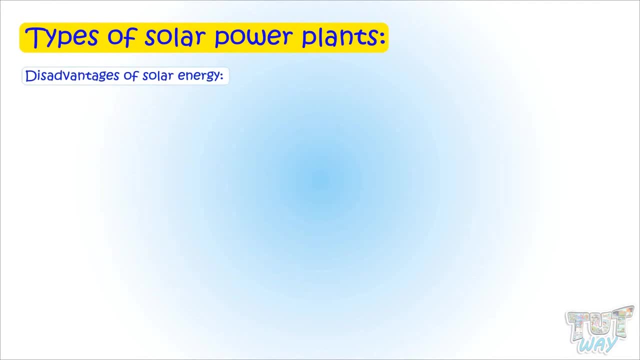 Let's learn the disadvantages of solar energy. Solar panels can generate noise. Now let's learn the disadvantages of solar energy, Solar panels and electric daddies. First and foremost disadvantage is that Solar energy cannot be created during the night time. Power generation is reduced when it is cloudy. 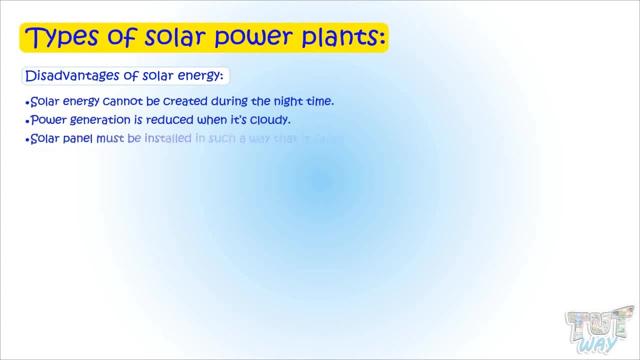 The solar panels are the light of life With the use of solar panels. solar panels are Weil light when they put out electricity. In other words, they are used to produce electricity and power by새. The solar panels must be installed in such a way that it faces the sun, so light they 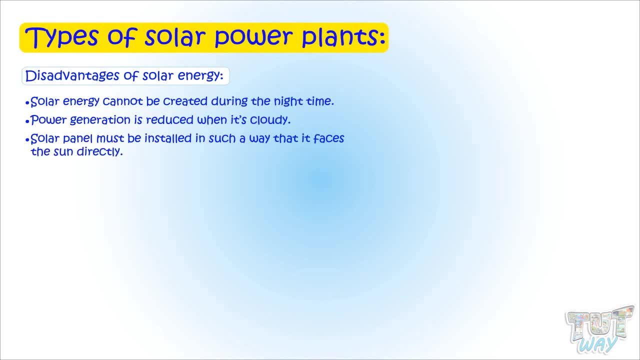 bring the energy out throughout the city. Solar panel must be installed in such a way that it facing the sun every day. There is sun in every one of these areas that manifest electricity- the Sun directly. Even most efficient solar cells only convert 20% of the. 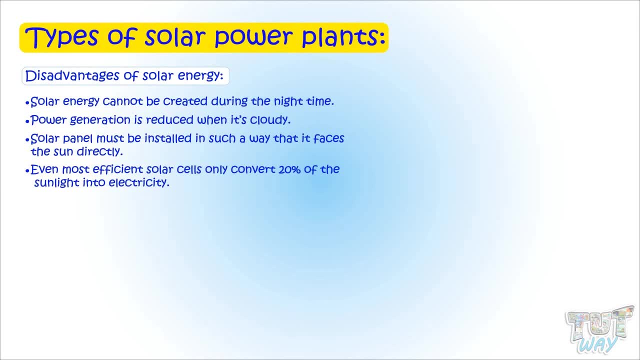 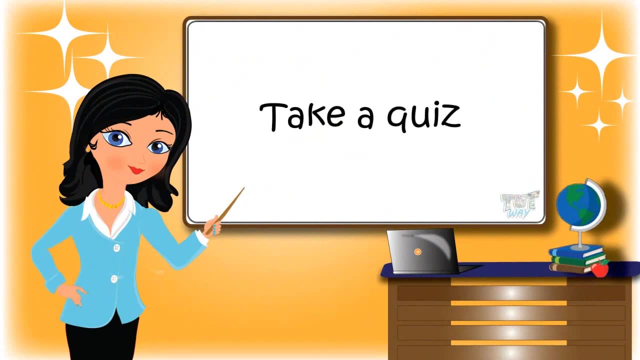 sunlight into electricity. Now you may go ahead and take a quiz to learn more. Bye-bye.